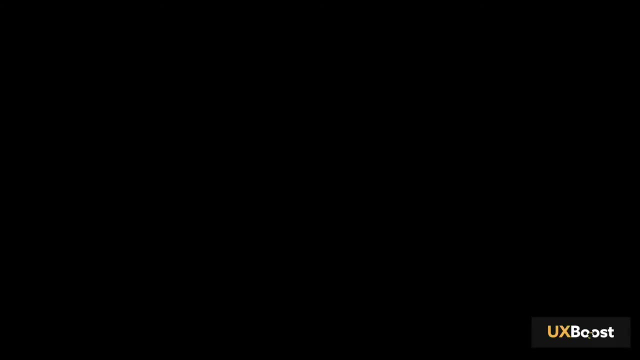 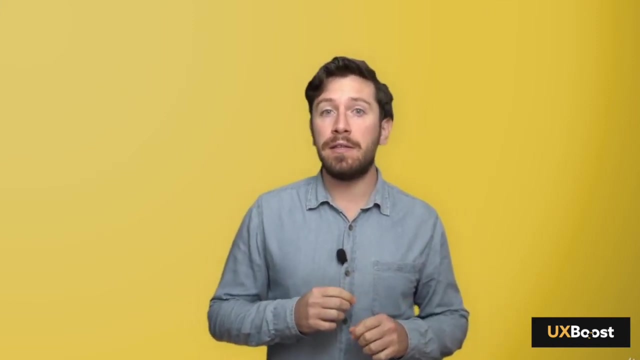 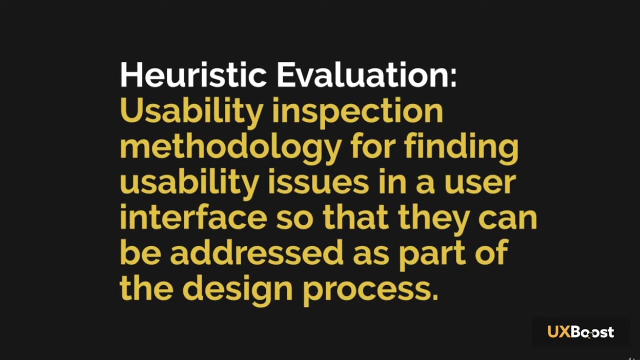 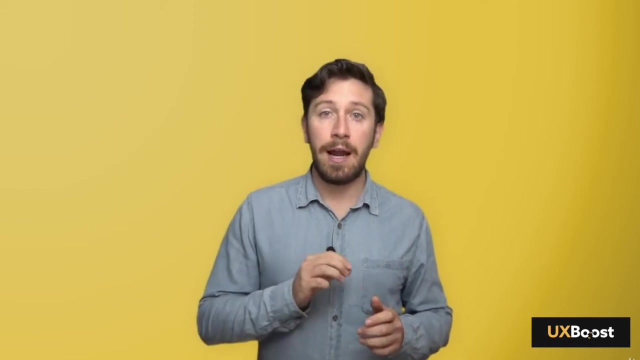 So let's learn more about heuristic evaluation. A heuristic evaluation is a usability inspection method for finding usability issues on a user interface in order to address them and solve them as part of the design process and the product lifecycle. A heuristic evaluation involves a small set of reviewers which examines the user interface and analyzes its compliance. 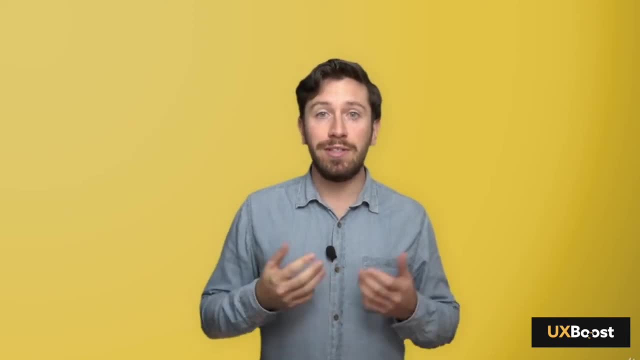 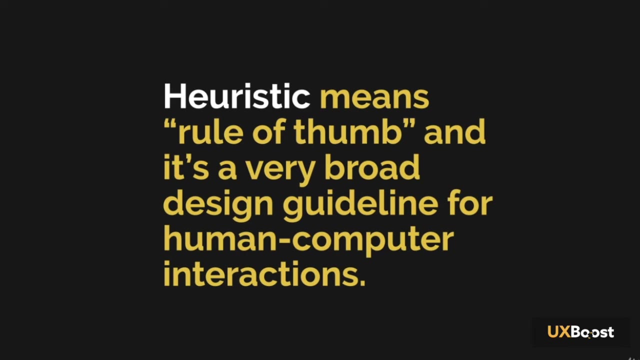 with 10 recognized usability principles, which are called the heuristics. Heuristic means rule of thumb, and it's a very broad design guideline for human-computer interactions. So it doesn't matter if it's a desktop computer, a mobile phone or you are designing an interface. 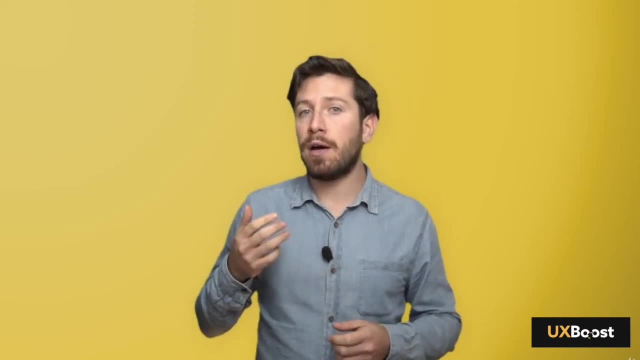 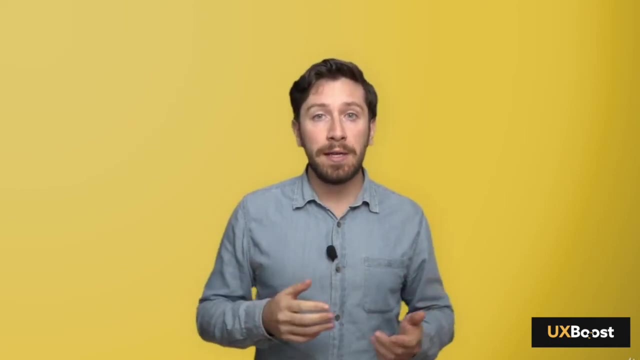 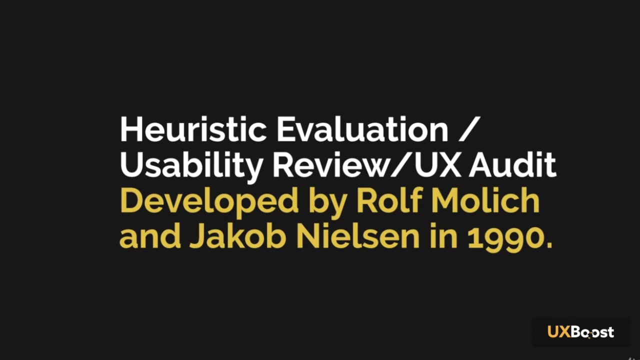 for a smartwatch. Also, it doesn't matter if you are working for a design for a video game, a website, an e-commerce or a software. These principles are broad enough to be applied to every type of user interface. This method is also known as usability review or UX audit, and was developed by the usability 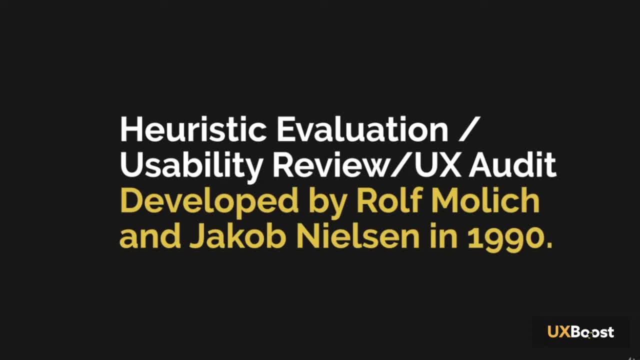 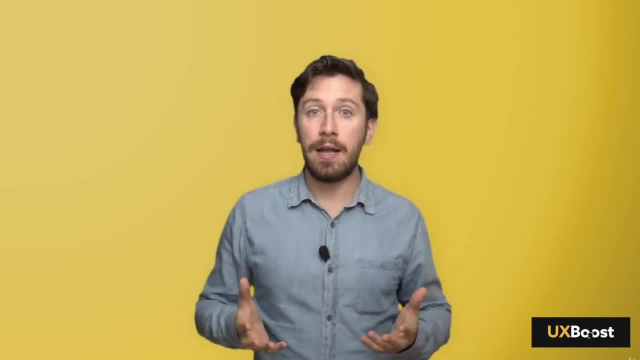 expert, Rolf Mollitsch and Jakob Nielsen in 1990.. The 10 heuristics did not change for more than 30 years and that's because they are broad design guidelines which comes from the basics of human behavior and interaction design. 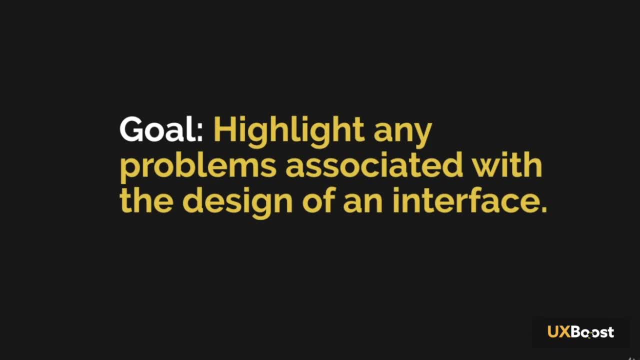 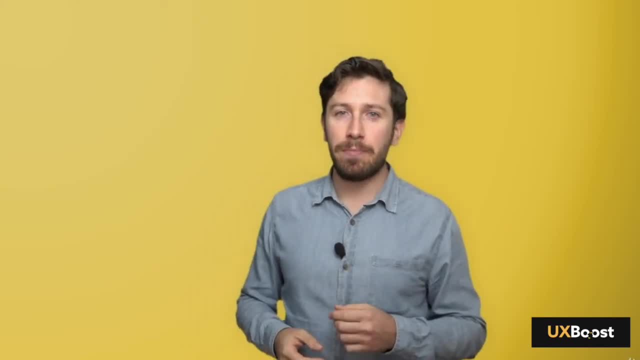 The main goal of heuristic evaluations is to highlight any problems associated with the design of an interface. Heuristic evaluations are one of the most important aspects of the design of a user informal usability inspection method, and it's particularly useful for those team which don't have a budget for user research activities or don't have a UX. 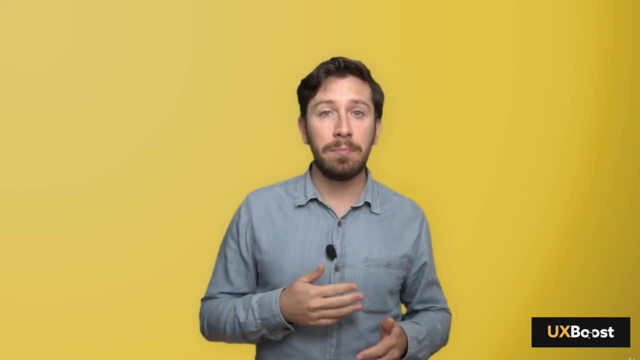 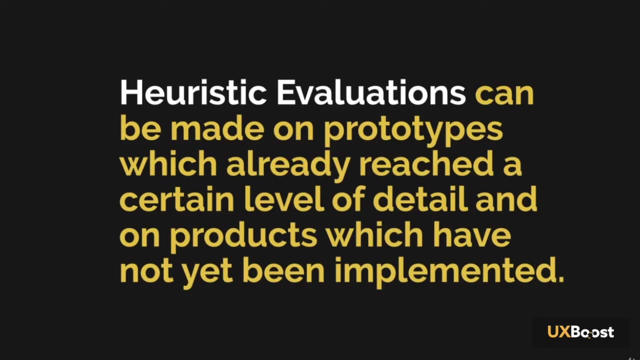 expert in house. With a heuristic evaluation, they can start building a product which, since the beginning, is respecting the ten principles of usability. Heuristic evaluation can be made on prototypes which already reached a certain level of detail and on products which have not been implemented yet. The simplicity and effectiveness of heuristic evaluation is very 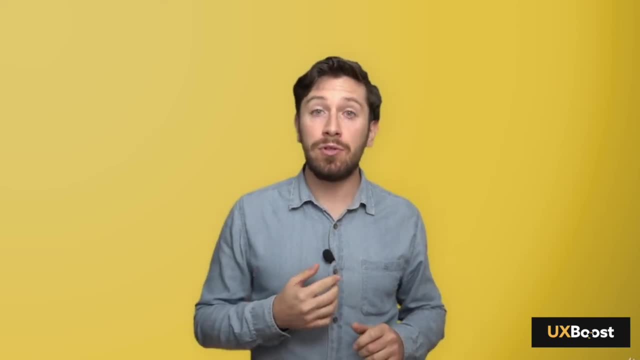 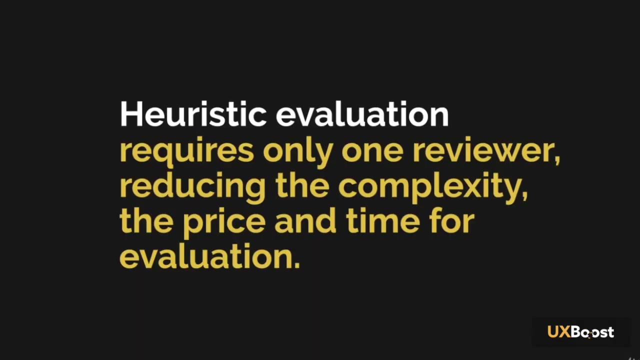 beneficial at the early stages of design. This method does not require user testing, which sometimes can be burdensome due to the need of users and a place to test. Heuristic evaluations requires only one reviewer or a small set of reviewers, reducing the complexity, the price and time for the evaluation In